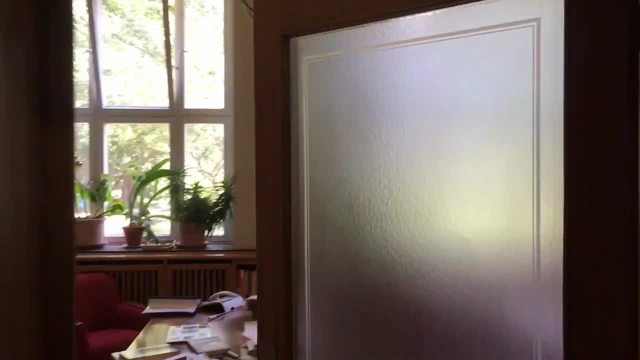 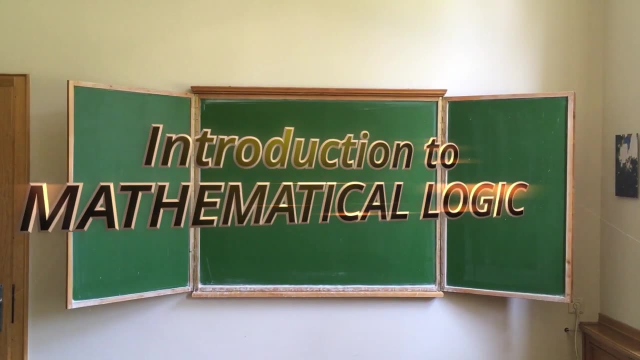 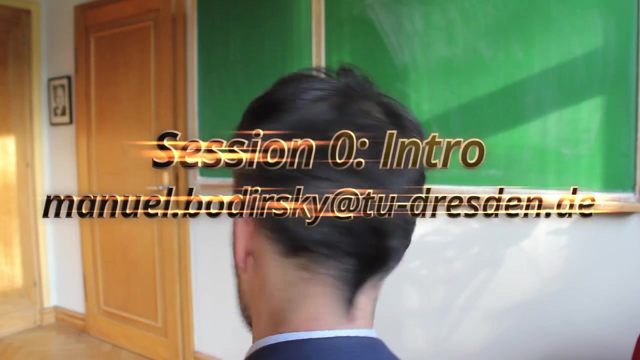 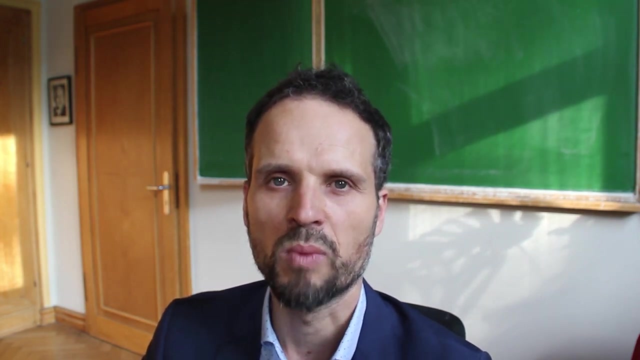 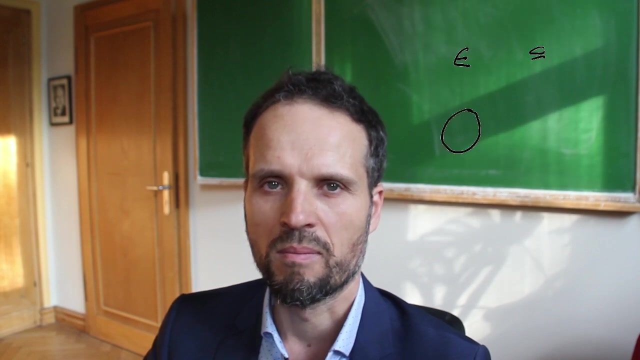 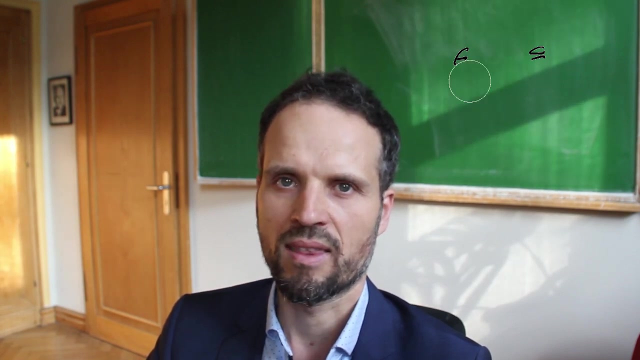 Hi, this is video material for the course Introduction to Mathematical Logic at TU Dresden. The target audience are mathematics bachelor students in their third year and diploma computer science students with a minor in mathematics. The prerequisites are some familiarity with basic set theory, As opposed to axiomatic set theory. this is also sometimes called naive set theory. 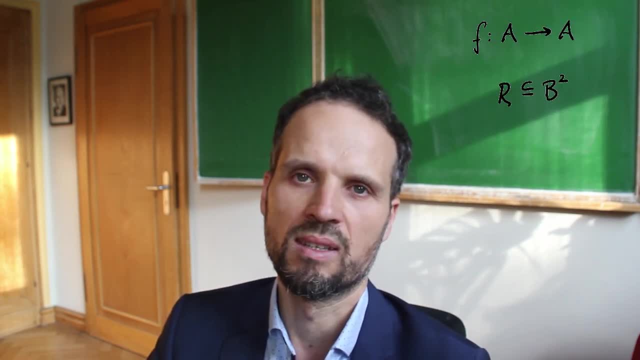 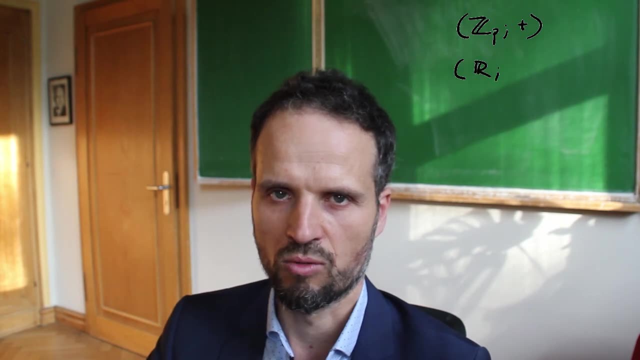 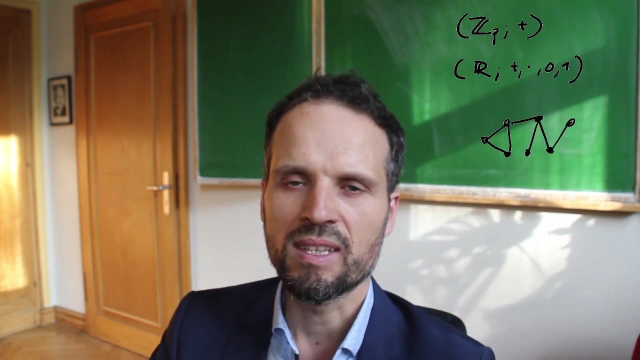 So I assume that you know what a function is and what a relation is. Ideally, you also know some fundamental algebra, Like structures such as groups, rings, fields or relational structures such as graphs and partial orders. We will need them as motivating examples for the more general concepts that we learn in 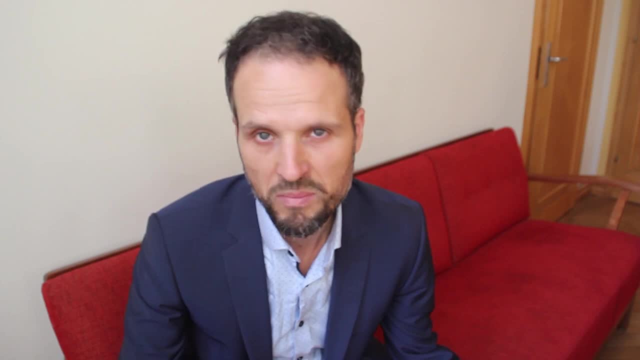 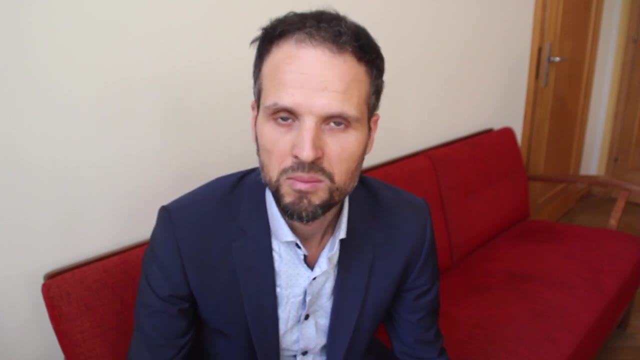 this course. These videos are just supplementary material for the course. The most important document of the course is the script, which will be made available chapter by chapter on the webpage of the course. The script also contains exercises. This is important. Doing the exercises is essential for succeeding in this course. 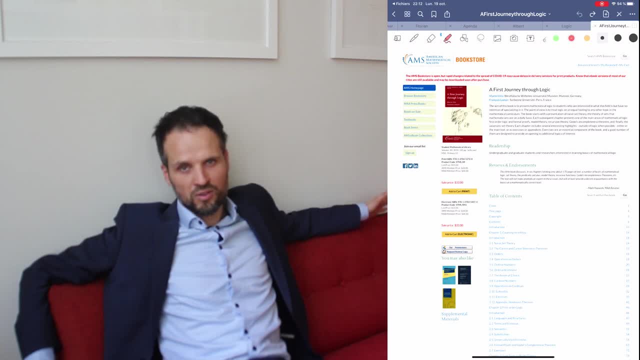 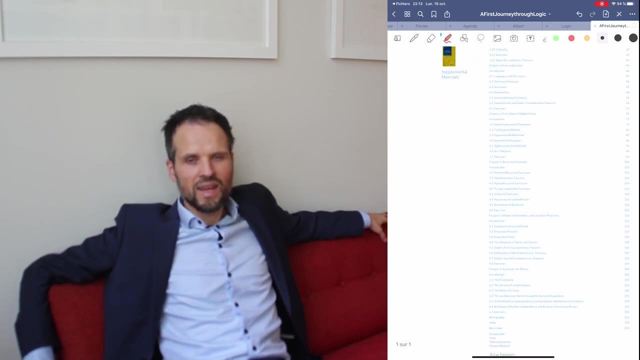 There is also a new beautiful textbook on the topic. It is called A First Journey Through Mathematical Logic and it's written by Martin Hills and François Lezer, published by the AMS. It costs 33 dollars And I can really recommend this book. 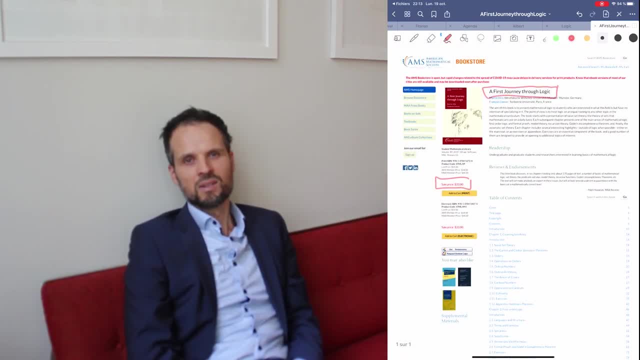 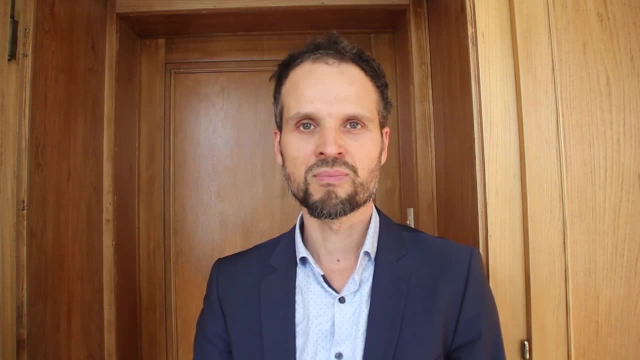 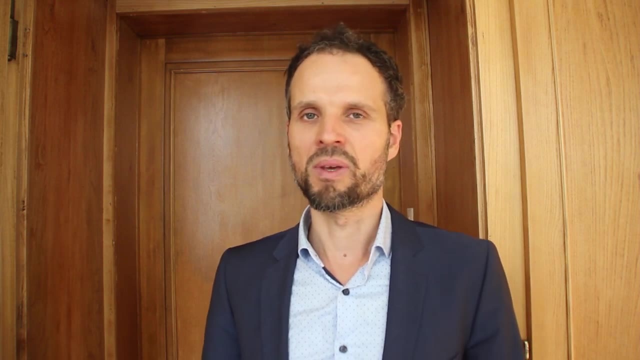 It provides a neat and optimized access To the subject. My name is Manuel Bodirsky. I am professor for Algebra and Discrete Structures at TU Dresden. Mathematical logic is a fantastic tool for me and in this course I hope to share some of my passion about the topic with you. 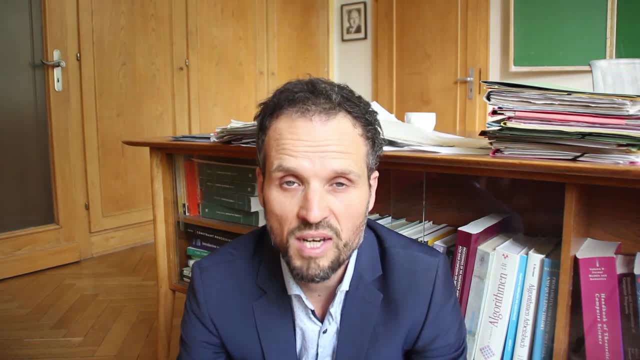 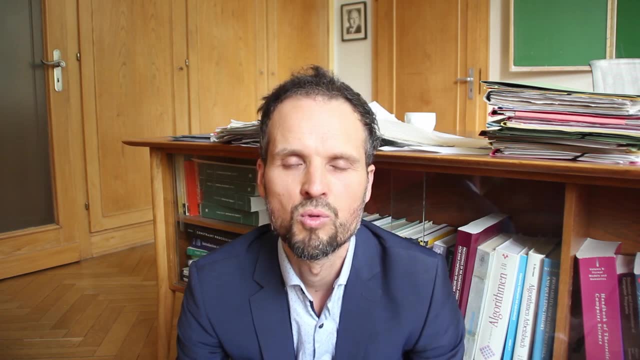 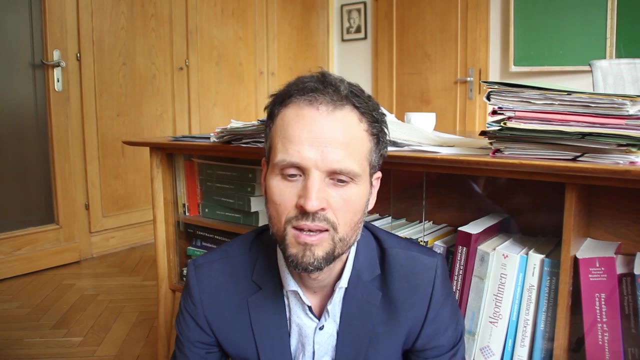 Today's video is about a motivation for the subject and also an outline of the content of this course. What is a proof? Proofs, Proofs, Proofs, Proofs are very much at the center of the mathematics curriculum at university, not. 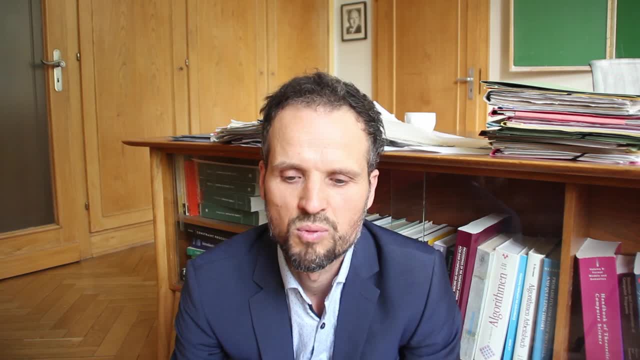 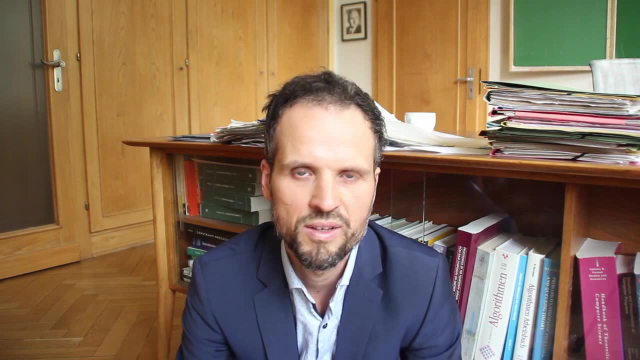 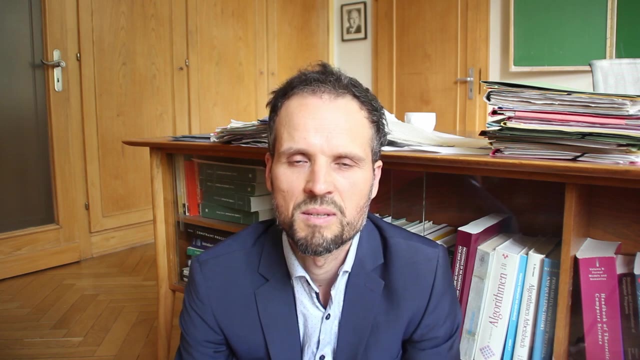 so much at school. So what is a proof? One could say it's a rigorous argument that convinces the audience or the readers that some statement is true. But what does it mean? convince? Convince who? Unconvinced, Unconvinced? 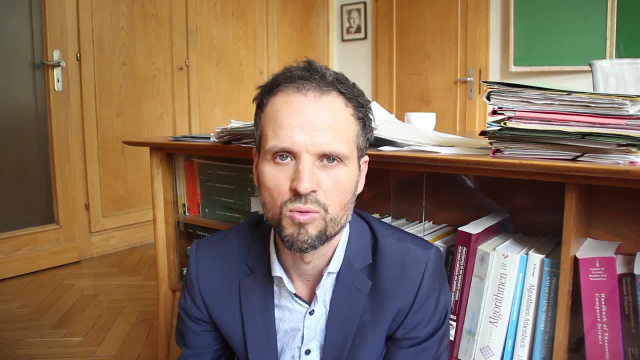 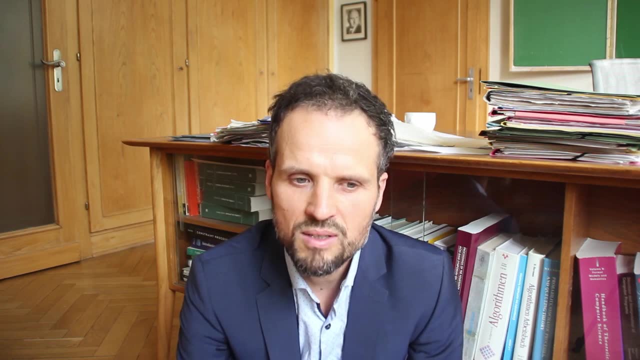 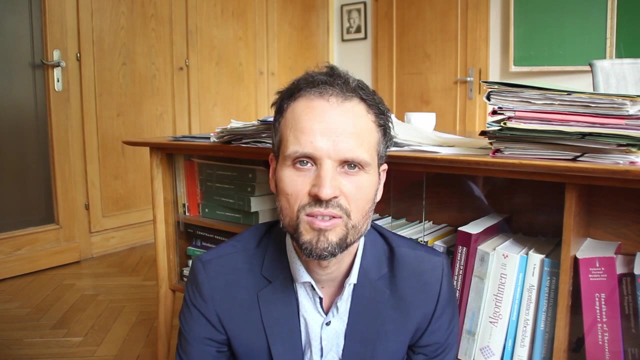 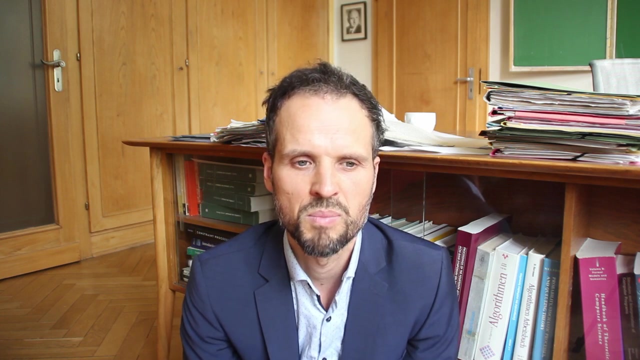 Unconvinced. Convinced who? the concept of proof, and we usually don't teach this in the beginning of the university program because it's actually technically demanding and it's not the most intuitive topic we start. we prefer to start with concrete topics because 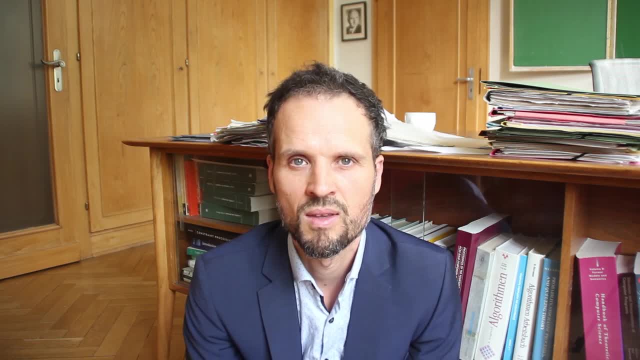 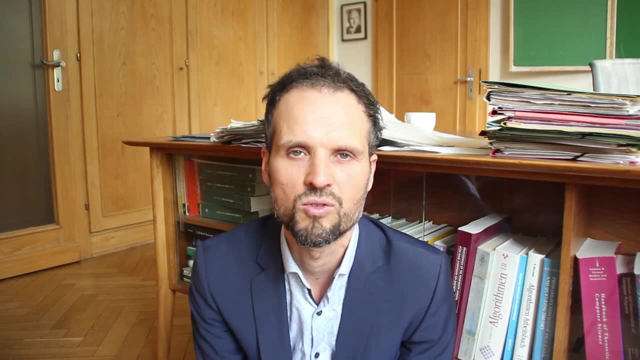 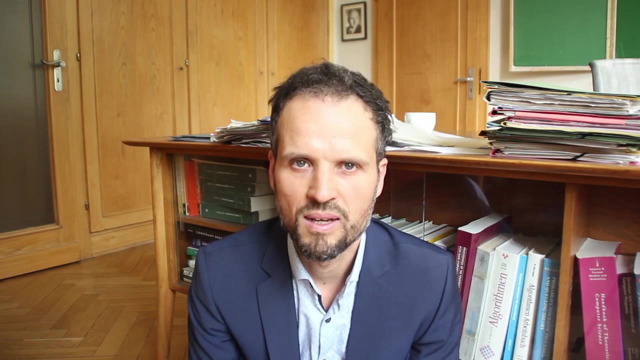 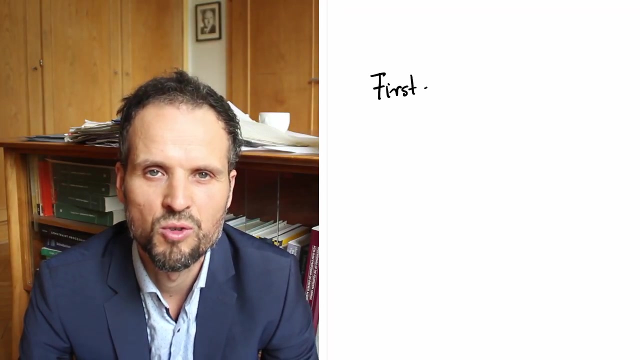 this is what students find easier. so what, precisely, is what constitutes a proof? what axioms are we allowed to use? precisely, what is a valid proof? step: this will be an important topic in this course. to formalize the notion of a proof, we need to introduce logic more specifically. we'll introduce, we'll work. 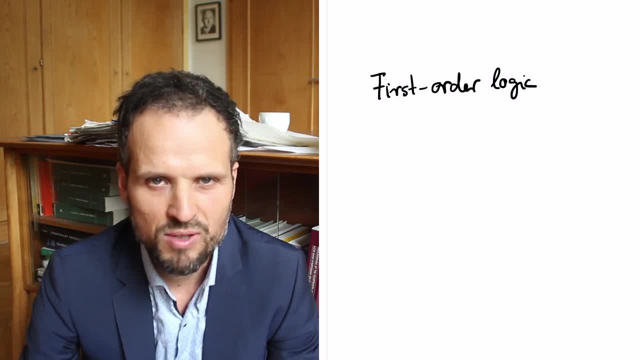 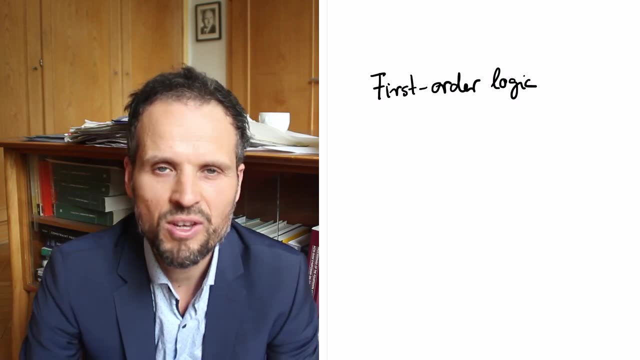 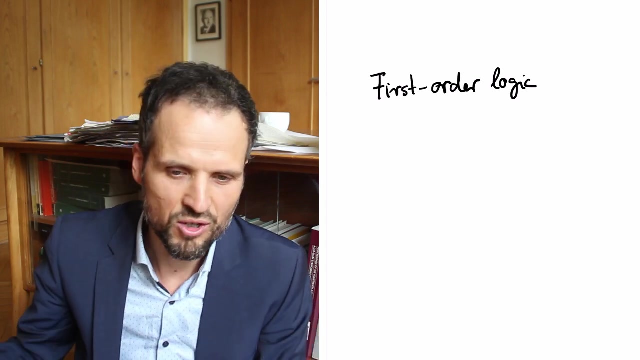 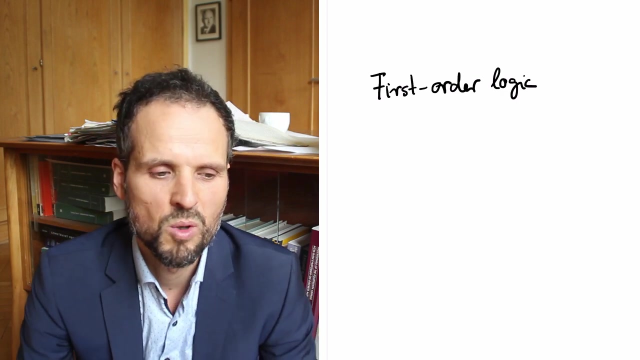 with first-order logic. first-order logic is in many respects the most important logic, both in mathematics and in computer science. it strikes a very good balance between expressiveness on the one hand side and very good model theoretic properties on the other hand. so by what do I mean by expressiveness? we can use first-order. 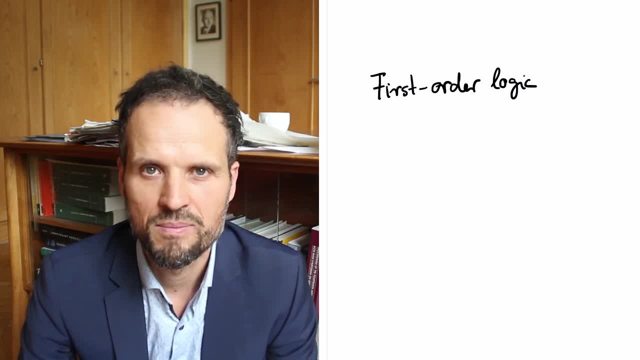 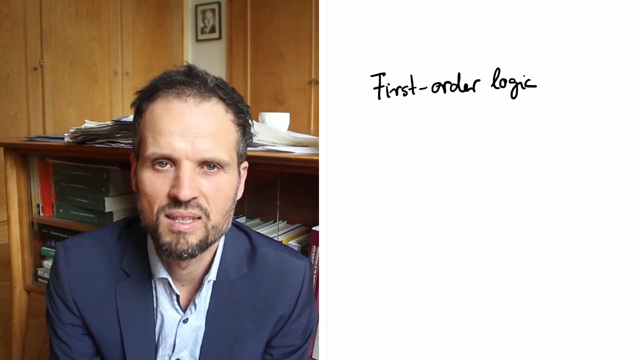 logic to formulate the axioms of first-order logic, to formulate the axioms of axiomatic set theory, and in this way we can basically perform all mathematics. we can formalize all mathematics within the first order logic. we'll learn this, we'll see this in detail in the course, by introducing Tzermelo-Frenkel set. 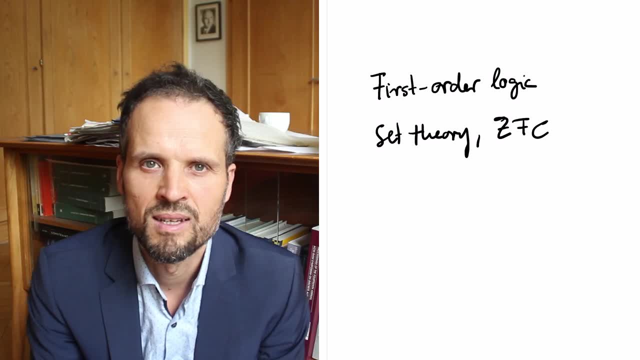 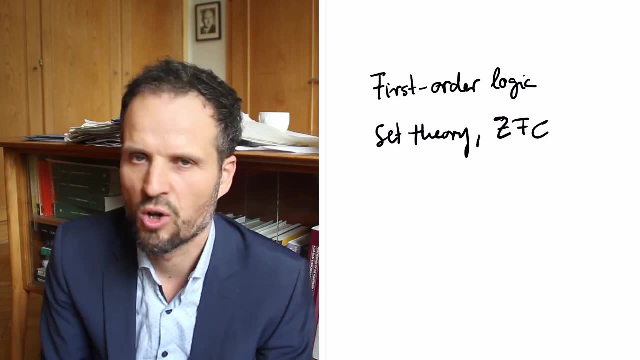 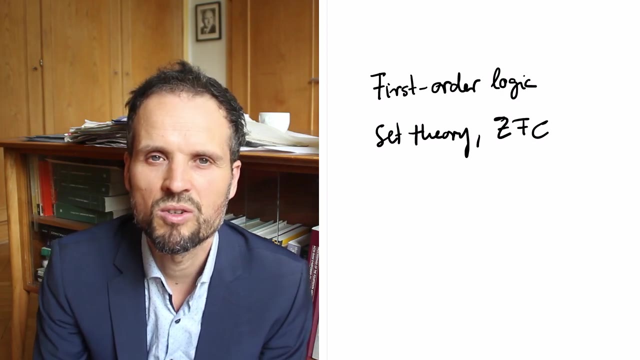 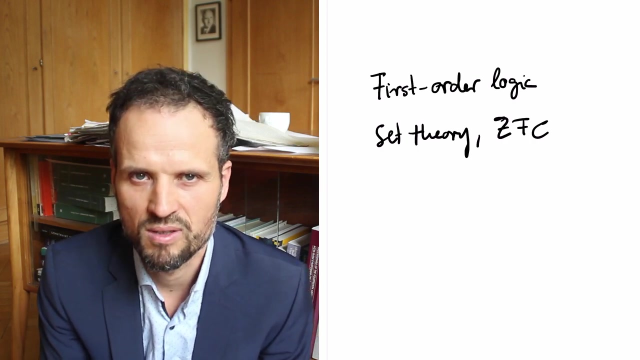 theory with the axiom of choice. this is sometimes abbreviated ZFC. you might have heard this already- And in ZFC we'll illustrate that you can code mathematics and we'll illustrate this with ordinals and cardinals. In what concerns the good model theoretic properties, I will have to refer to the model theory courses. 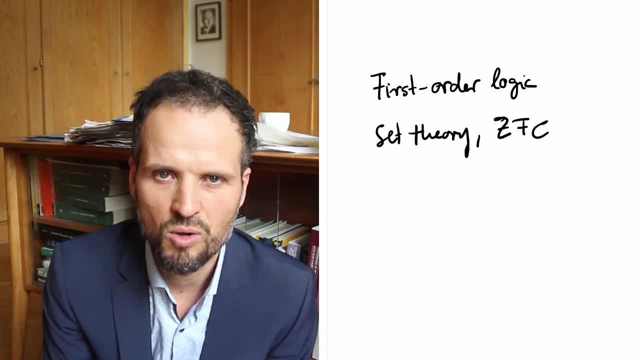 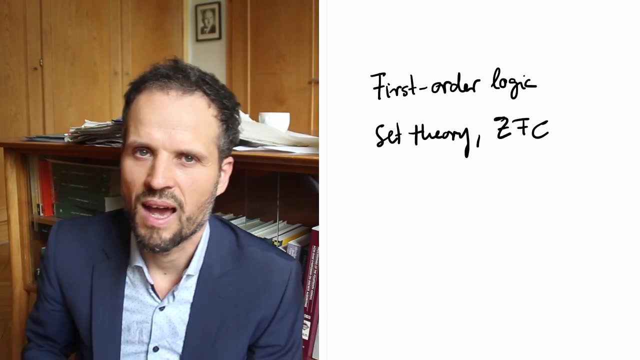 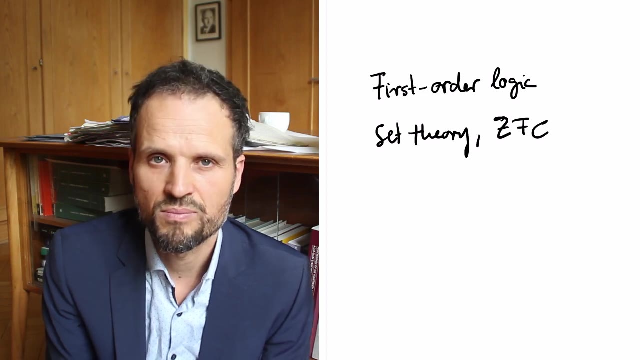 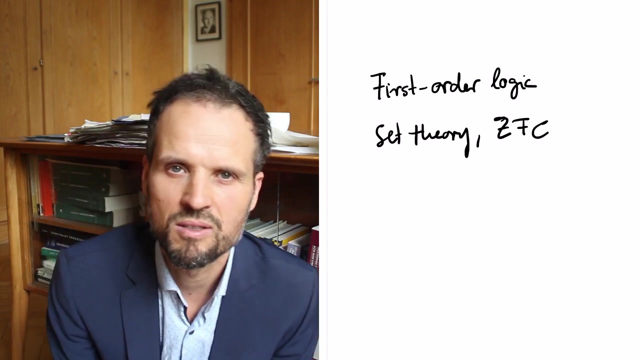 This is maybe outside the scope of this course. In computer science, in many applications you study either extensions of first-order logics or restrictions of first-order logic. First-order logic itself is already important. It basically corresponds to the most common database query language and many restrictions and 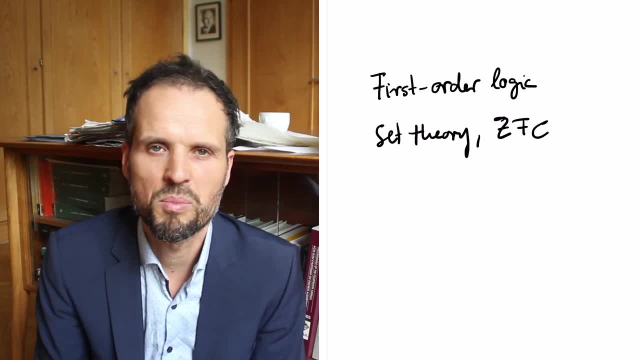 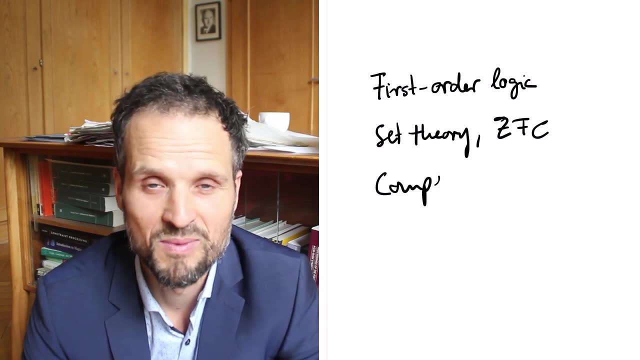 extensions are important, but this basic starting point is always first-order logic. So it's really central in computer science. The first bigger goal of this course is to study the first-order logic. The first bigger goal of this course is to know the first-order approach and to get started running the tool. 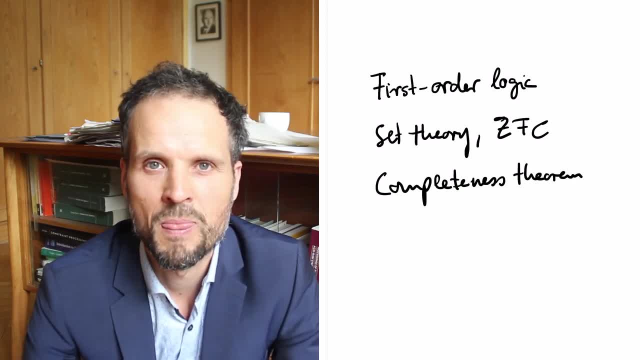 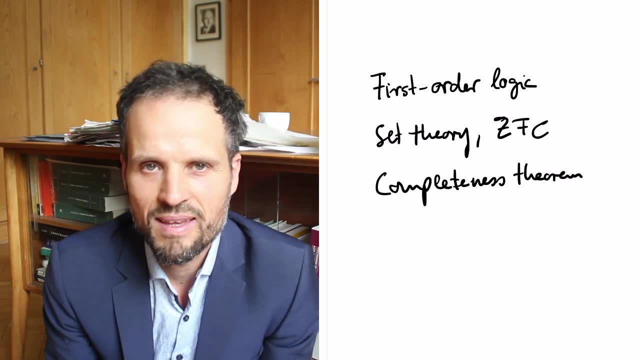 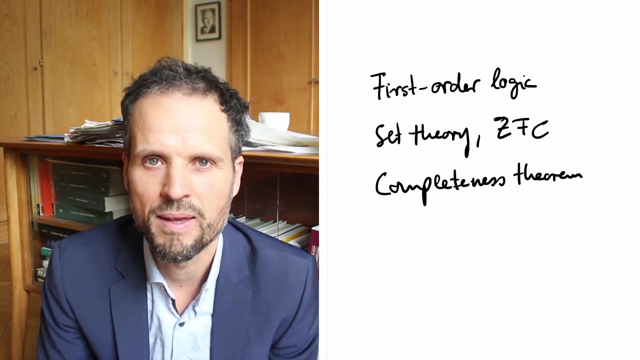 Now there is a fundamental sculpting need to be done in order to sew the inflar fireworks up inside the Nevada Park, And the first couple of things we'll do are first-order economics. We may well 지금 start with instruments and 가ussman probes, because then you get. 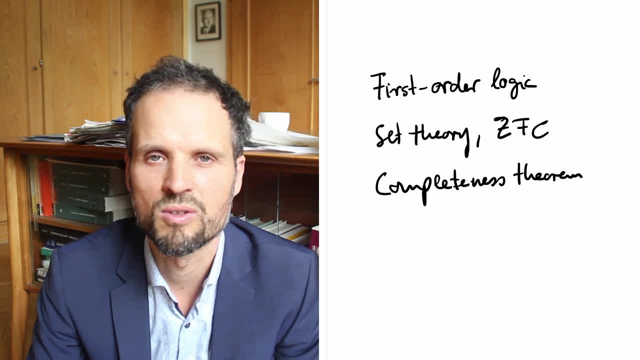 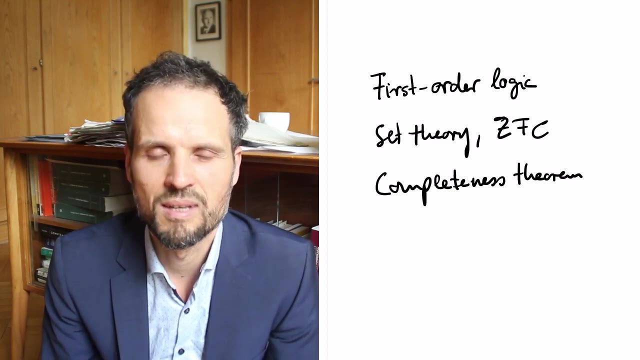 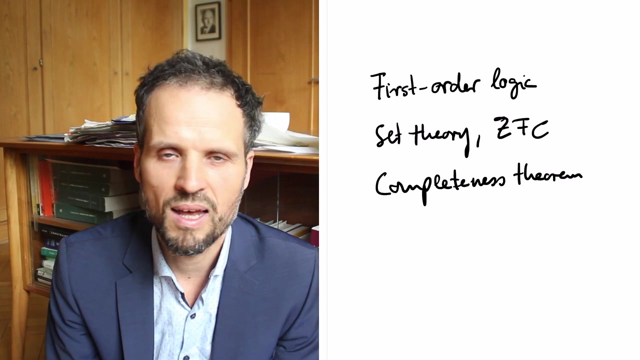 to know how the field is happening. property of our notion of formal proof is that all valid statements have a formal proof. And the third important property is that this proof system is so simple that we can program a computer so that it recognizes all axioms that we are allowed to use in these proofs. 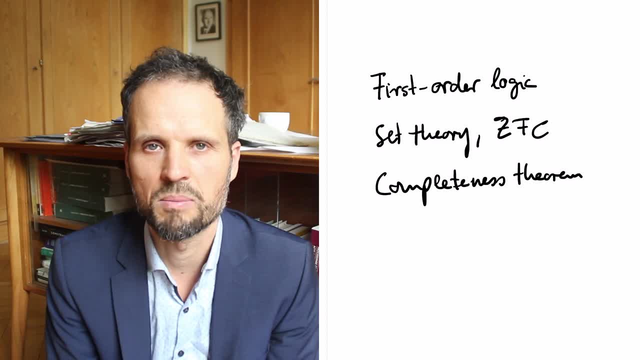 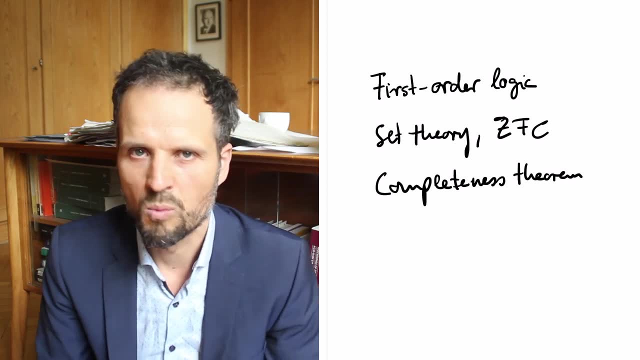 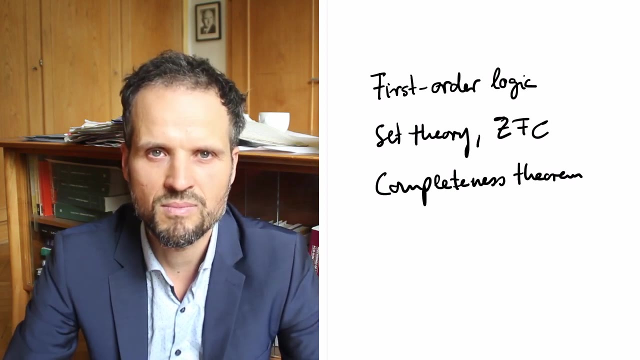 and the computer can also check valid proof steps. Valid proof steps are very simple and by combining the axioms with these very simple proof steps we can prove all sentences in mathematics that are true. And this is Gödel's completeness theorem, and it has many remarkable. 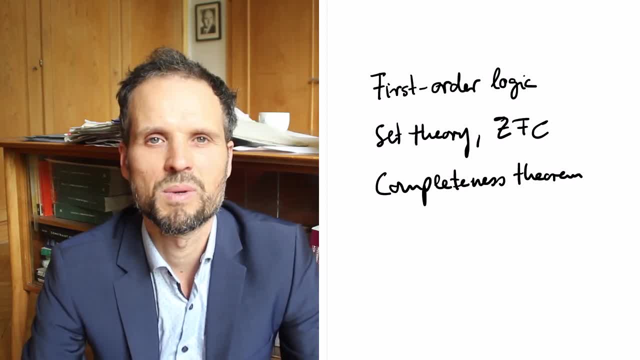 mathematical consequences. The first one is that we can use it to prove the compactness of a sentence. The second one is that we can use it to prove the compactness of a sentence. The third one is that we can use it to prove the compactness of a sentence. The fourth one: 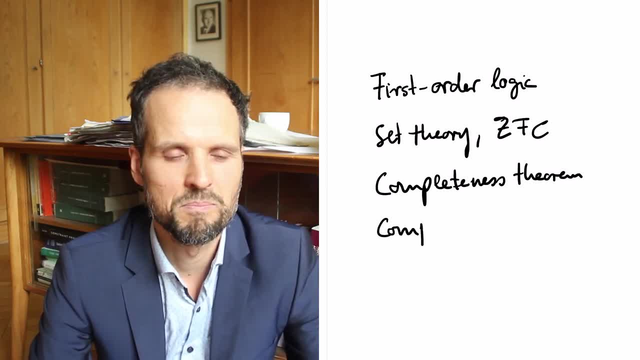 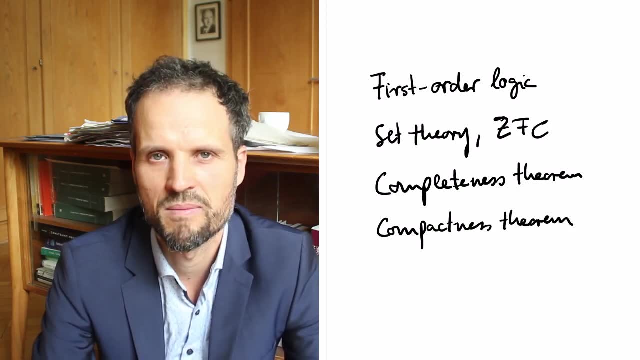 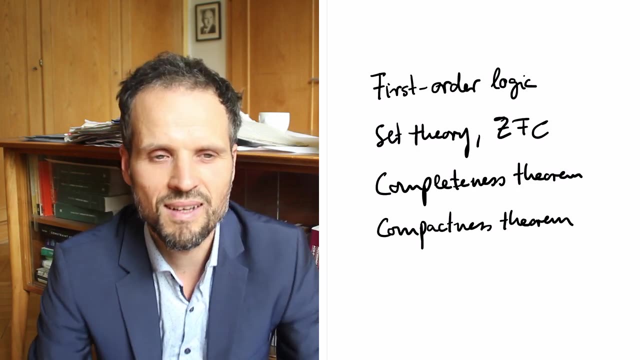 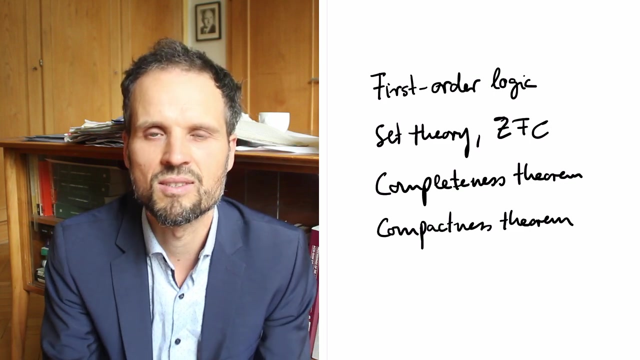 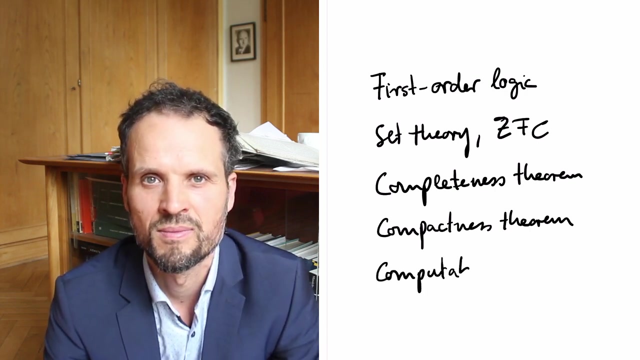 is that we can use it to prove the compactness of a sentence. The fifth one is that we can use it because we can't replicate this on a single element of our reading. And finally, proofs. but in fact this also means that we can program a computer to find proofs. 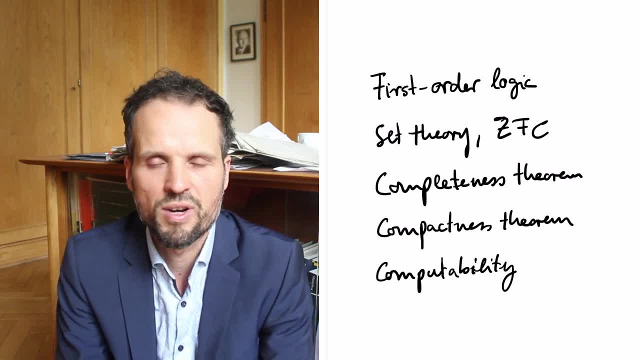 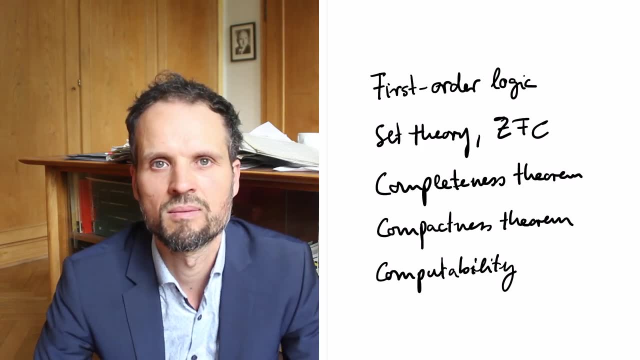 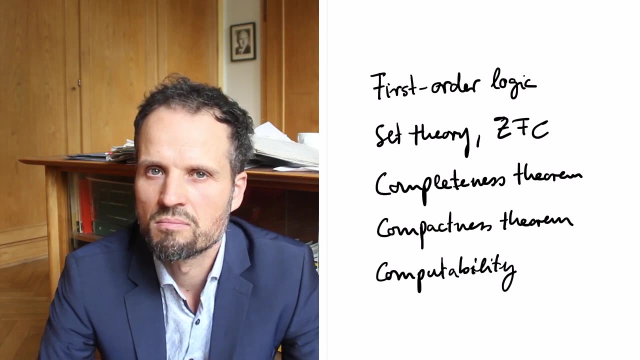 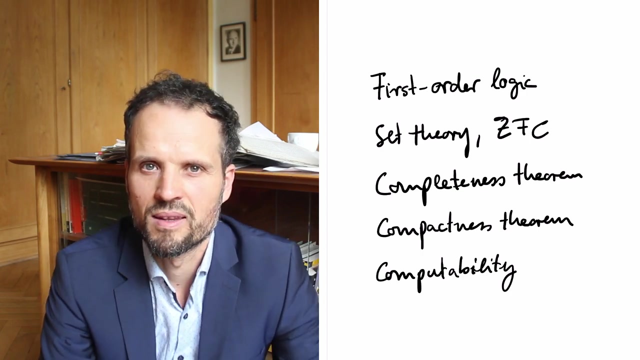 because we can simply list exhaustively all strings, all candidates for correct proofs, and then check whether they are correct. this is of course not a very efficient procedure, but it also appears to be a computer science issue. but in fact it has a very remarkable mathematical consequence one can use. 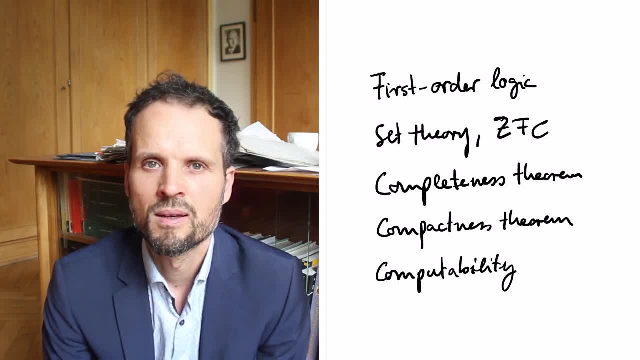 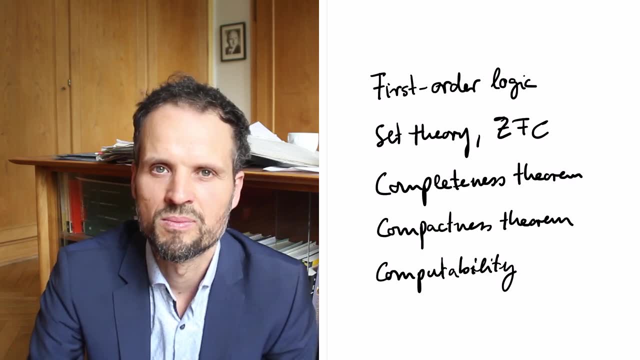 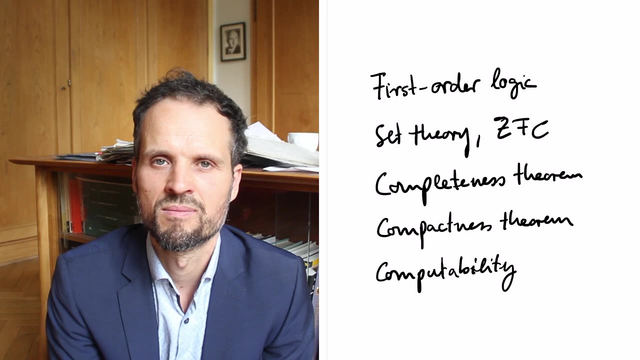 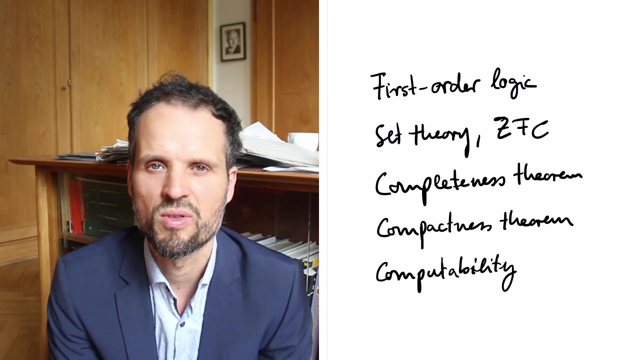 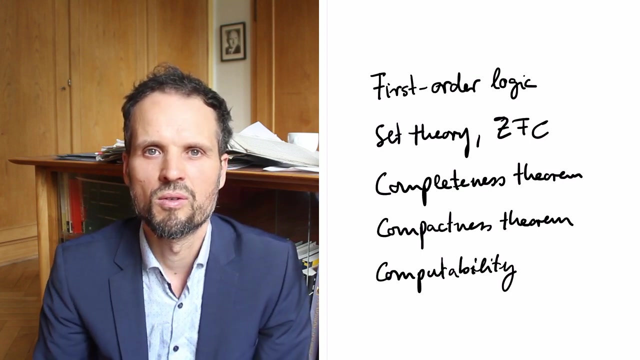 this to show that there are statements which don't have a proof and also their negation does not have a proof in ZFC. so these statements are independent from ZFC and this is nothing special about ZFC. in fact, one can show this for all theories, for all axiom systems that are expressive enough to formalize a 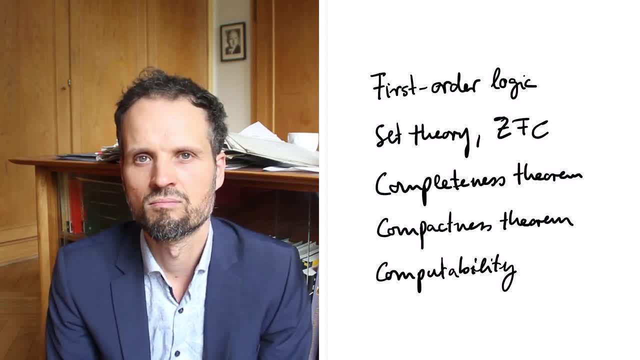 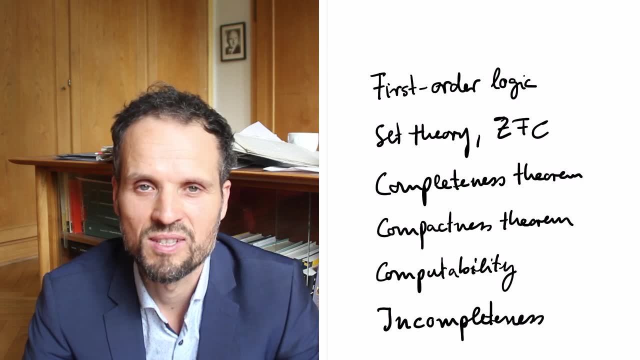 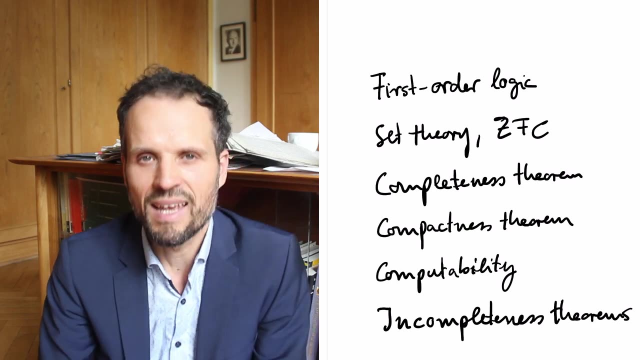 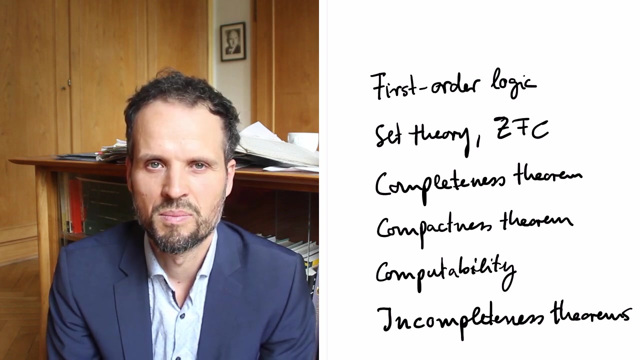 sufficiently strong part of arithmetic. this is called Gödel's first incompleteness theorem. and in fact something more is true, something stronger is true. one can even show in ZFC that there is no proof in ZFC that ZFC is considered true. Being consistent means you can't derive a contradiction from it. We would like to be consistent. If we would be inconsistent, everything would follow from the axiom system would be worthless. So of course we want that ZFC is consistent. but we can't prove it in ZFC And this can be shown. 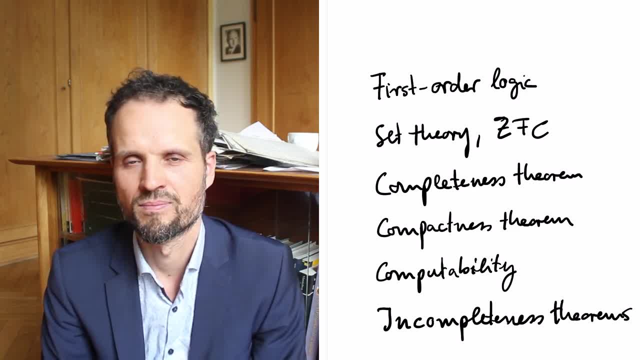 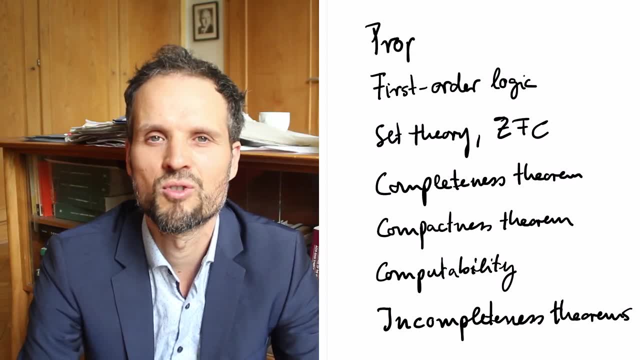 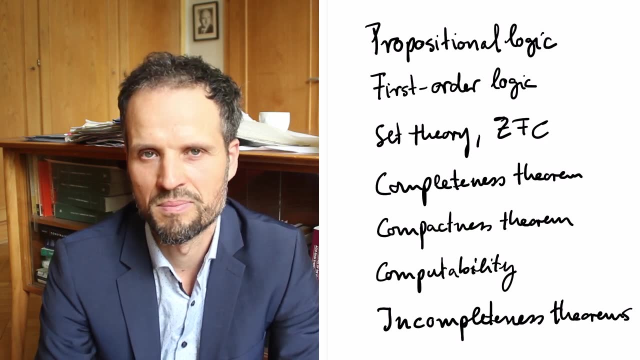 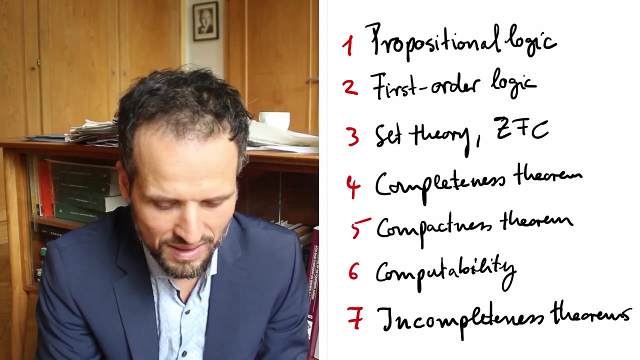 We can show that we can't show. But we'll start very slowly. Before even introducing first-order logic, I will introduce propositional logic. This is some sort of warm-up. Propositional logic is a microcosm of logic and it contains already many aspects and concepts. 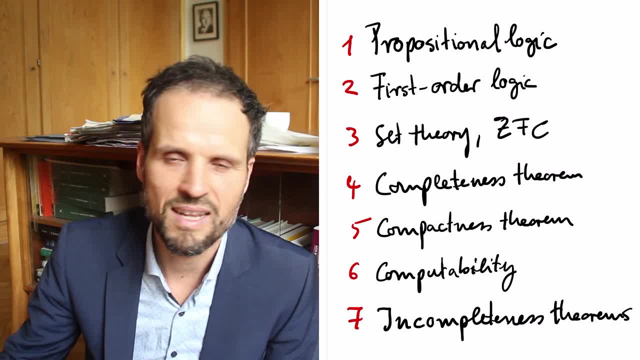 and ideas. So let's first practice a little bit with propositional logic.